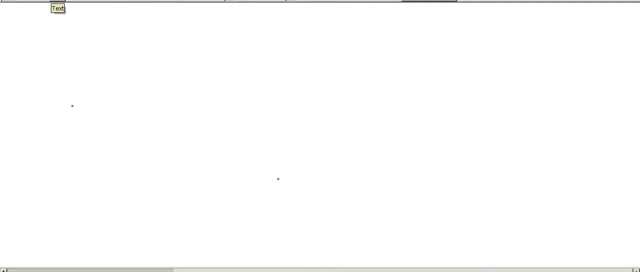 Hello, students, in this video lecture I will explain you the concept of finite automata, as well as the deterministic finite automata and all the tuples or all the elements it has in it, and what are the elements they make this deterministic finite automata And the notation is used in the definitions, with example, And it will surely going to help you understand the concepts of finite automata. This is the part 3 in the series of finite automata and these are the important topics that I have covered as far as the discrete mathematics. 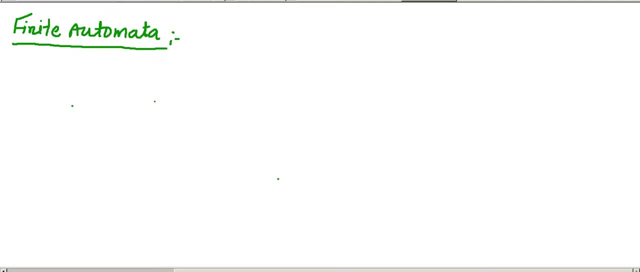 And it's concerned right. So let's start with the definition of finite automata. Finite automata consists of a finite memory called input tape Right. So it has a memory. It has a memory And it is known as a input tape Right Input tape. 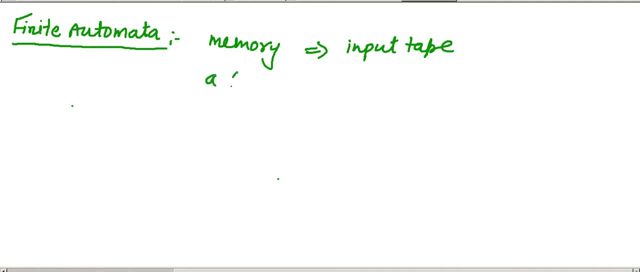 And a finite non Empty set of states. Finite non empty Set of states. Right, And we'll explain each of these things. Right. What is input tape and what do you mean by a state? state means in which stage or in which state you are Right. 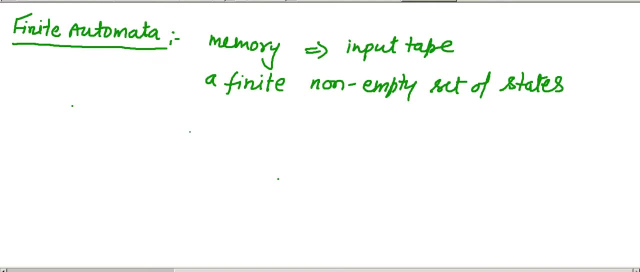 Okay. So if you take an example of a journey, So if you are going from point A to point B, then there are several points that exist between A and B. So these points are your states Right. So when you reach some point starting from A, you reach some point A1, then you move to A2. And finally, you are reaching to the point B. So these points are your states Right And the A is your state Right And the A is your state Right. 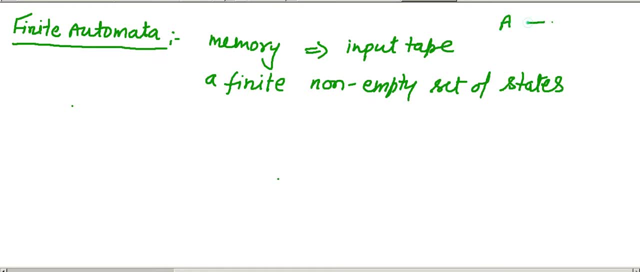 a is your, obviously. a is your initial state and b is your final state. so this was just an example to explain you the concept of states right now. what other it has means finite automata, right, so it has an input alphabet, right, and you know the alphabets. what are the alphabets and? 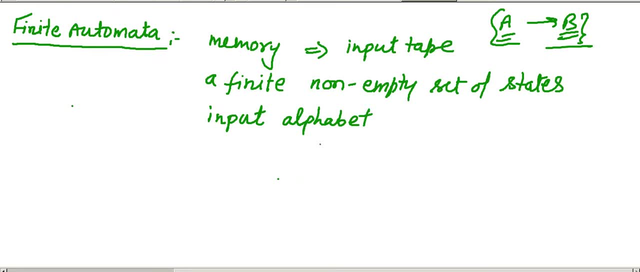 what do you mean by alphabetically? and this is nothing but a set of some symbols and denoted by this site. then it has a read only head, right, read only head and other things it has. it has a transition function, test transition function- right. then this is: this function is like this: it applies to these states and it decides that how these. 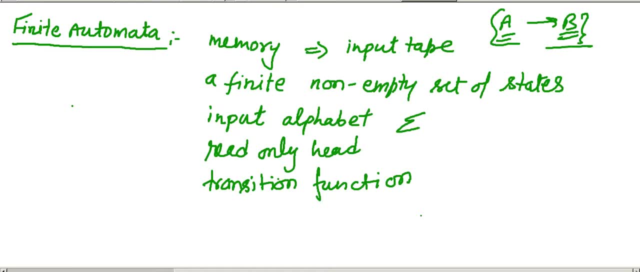 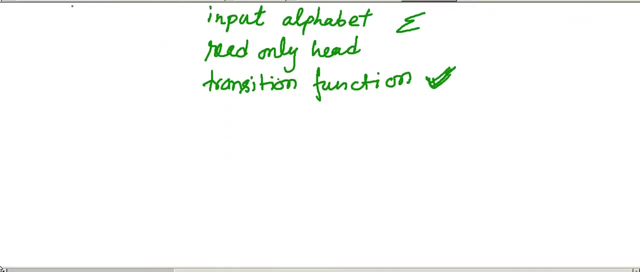 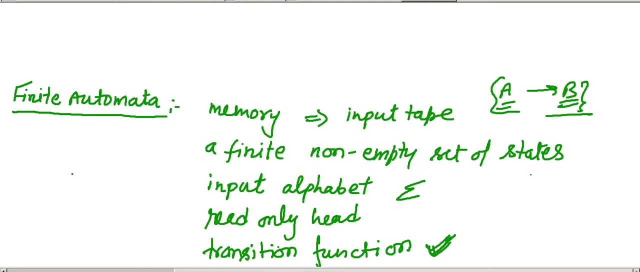 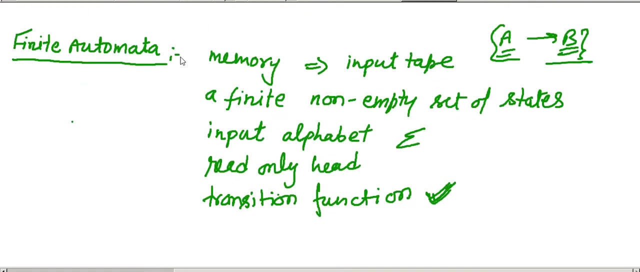 symbols, or how these points are, or these input in in in the input tape is moving from one point to other because of this function means so. so these are the basic things that means if it consists of all this, and this is known as finite automata. so these are the things that makes sorry, that makes the finite automata, so you can count. 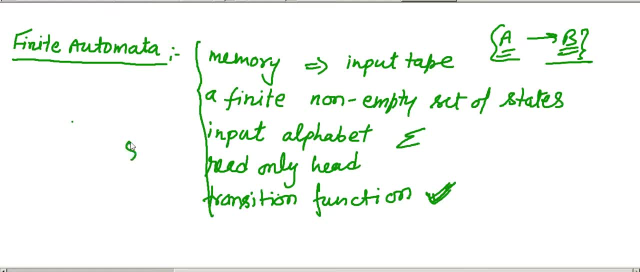 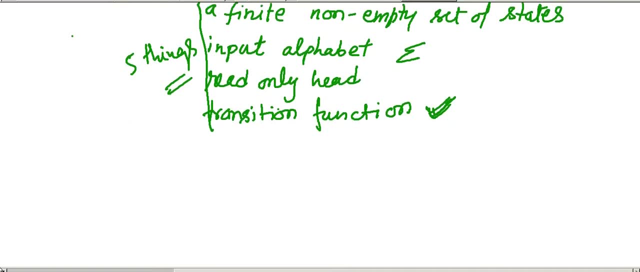 one, two, three, four, five. these are the five things, right, five things. so remember five things and these five things, and they have made the notations for, for representing these five, five steps, right, so we can consider it as like this: this is a, this is a tape, right. 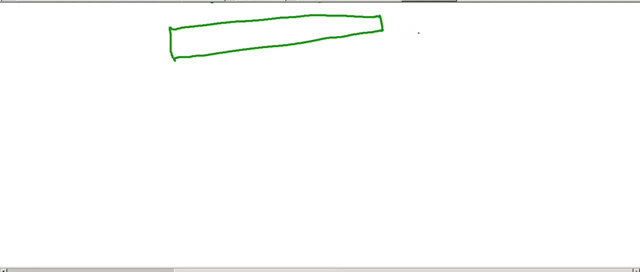 this is a tape, this is memory right, this is input tape. this is input tape and we have this, this is these. this tape, which is is a memory and it is divided into cels and, and this is a control, known as finite control right, fc, and it reads the these symbols that are stored: 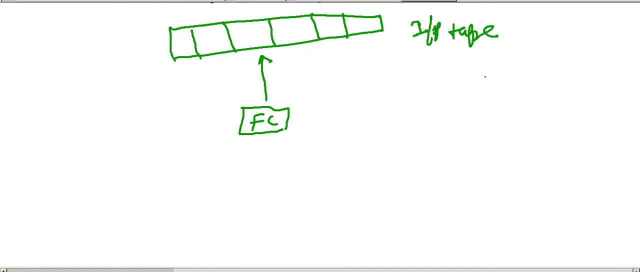 on this input tape and this is the basic model of model of finite automata: finite automata and, as in your booklets and and in various books, so the starting of the symbol, starting of the symbols by this sign and this is the final symbol which is stored on this input. 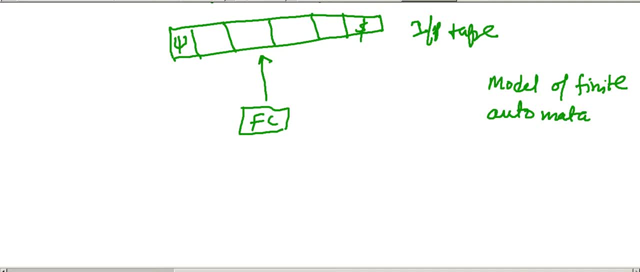 tape is uh shown as dollar right. so if they ask you in your exams about what do you mean by finite automata, so you you will define the finite automata by, by by saying that it consists of five things: which is the initial state, is the set of states. 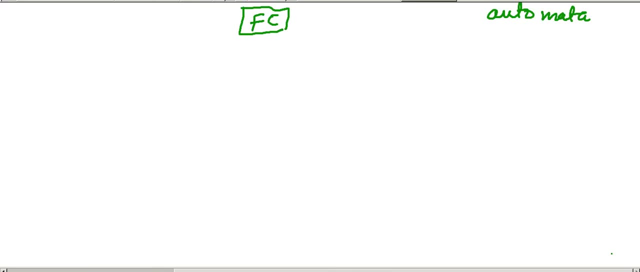 set of alphabets and a input tape and transition functions, right, a read only head and all that. so so what is deterministic finite automata? this is the general definition of automata, but the the. so what is deterministic finite automata? if you look for in your syllabus, then you will find that. 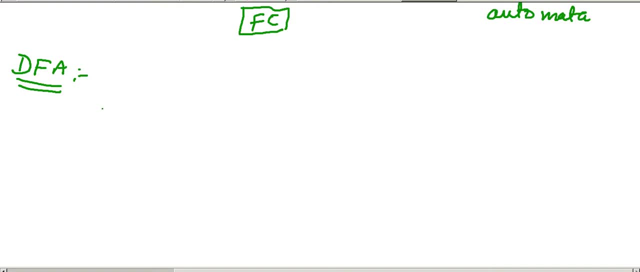 uh, they have asked you or they have explained the deterministic finite automata and if you read your booklets you will get to know. but okay, if you don't know about and you have not heard this term, what is our dfa or deterministic finite automata? so a deterministic finite automata described as a 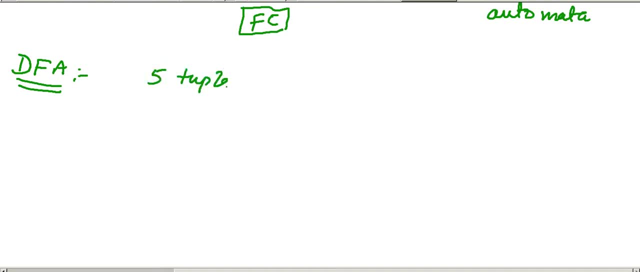 five double right this in one of the examples i will show you how that can interact with each other � bees are the examples. these are five tuples which represent alphabets and the cepal neighboring faltas five tuples represent all lines that are in the set of final states 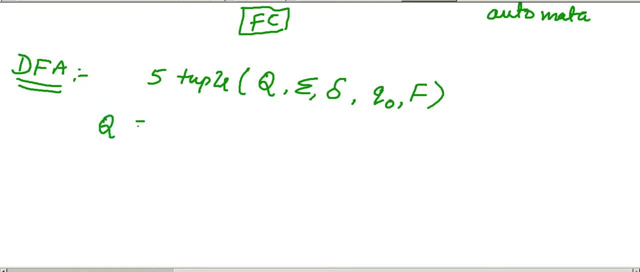 These symbols represent Q. Q represents the non-empty set of states. Non-empty set of states, So there are various states And this symbol is very much familiar to you. If you have watched my earlier videos, then this is nothing but the alphabet. 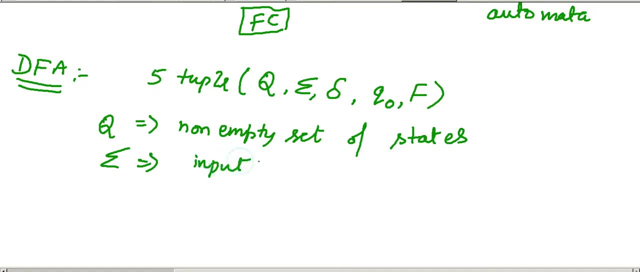 Input alphabet. Input alphabet. So these alphabet can be 0 comma 1.. Alphabet can be A comma B, Or A comma B comma C, 0,, 1,, 2 and whatever the alphabet they are using, And this is the transition function. It denotes. the transition function Means how you move or how the symbols move in this finite automata. 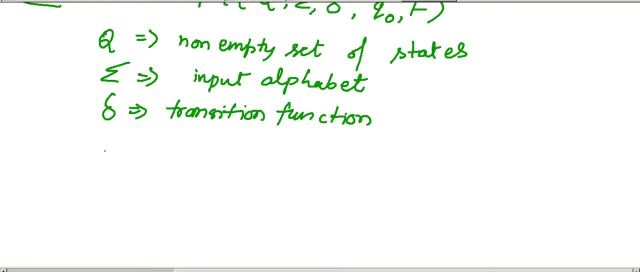 Then we have this: Q naught. Q naught is your initial state or starting state, Initial state, Right, And this is obviously belongs to one of the states which are in this automata Means Q is a superset and Q naught is a subset of this set, Right. So that's why we can say that Q naught is a subset of Q. 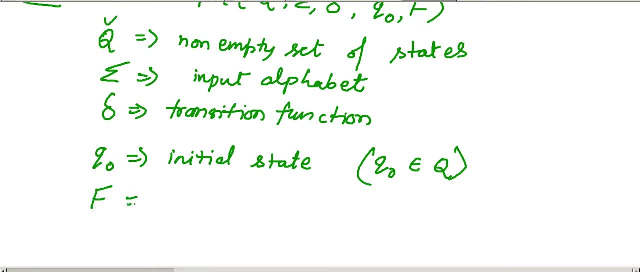 And then we have a F, Capital F, which is the set of final states. Set of final states, Right Final states Means finally, you are going to like, as I have taken this example- A to B, Then B is my final state. 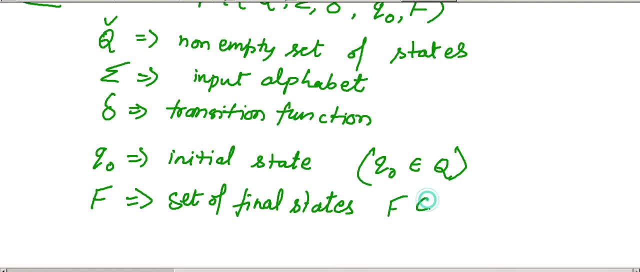 So this is also the subset of what Q, Because Q is the set of all states. So Q, naught and F are the states. Q naught is the starting and F is the final. We can say that F is a subset of Q. 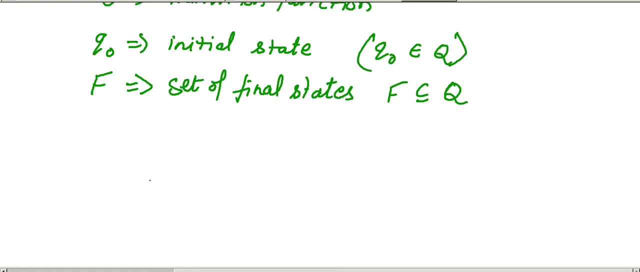 So how these notations are used and represent Right. So first, the notations that how these notations are used, Notations How these, because these are the symbols and but How they are denote How they are used to denote in a finite states, machines or whatever state machine. 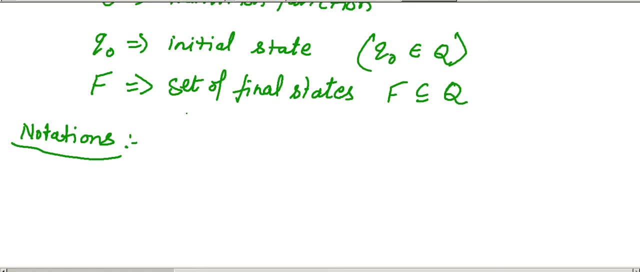 It is finite, It can be finite, It can be non-finite, It can be deterministic, non-deterministic, Right? So this is first thing that you must know, that how to represent this. So, initial state, as we know, The initial state. 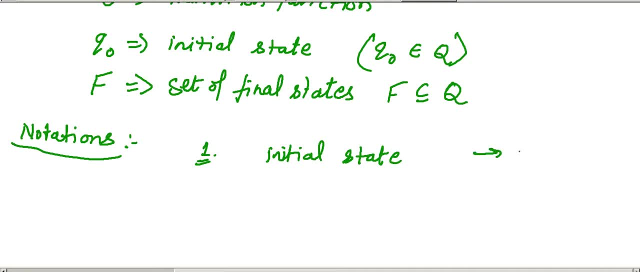 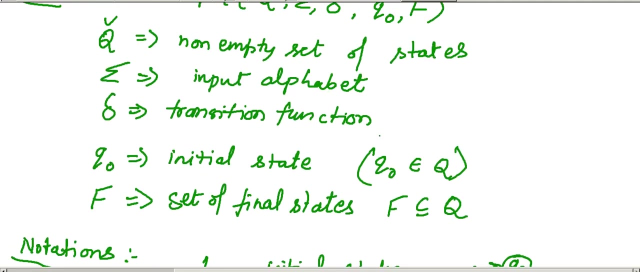 Is represented as this. So this is your initial state, Right? So we know the symbols. as I just told you that it consists of five things: Non-empty. set of states. Input alphabet Transition functions- Q- naught is your initial state. and set of final states. 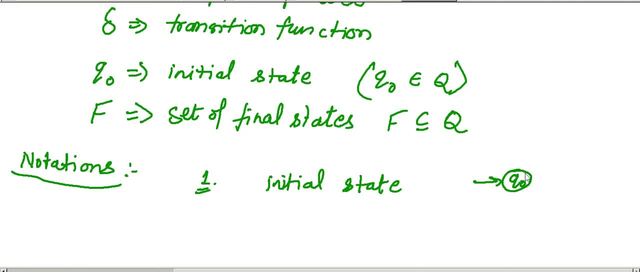 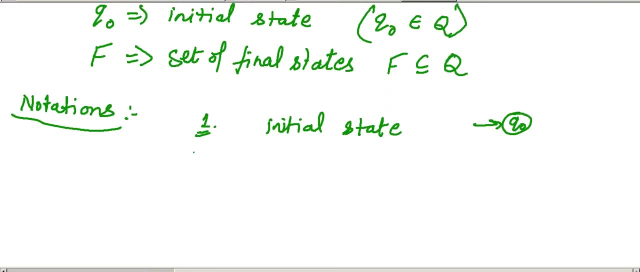 So in the diagram you represent like this: So this is your. if the arrow is before this state, Then this state Is initial state, Then the second is your final state. Right Final state is represented as the symbol using the double circle Right. 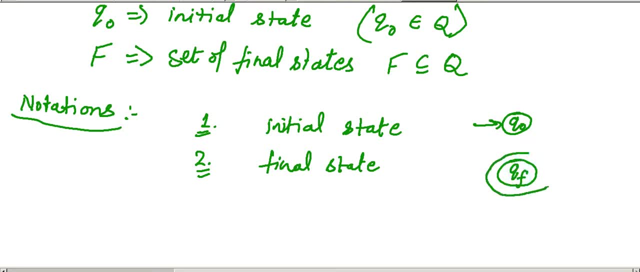 So we have this final state and Okay, So this represents the final state. Then we have a transition function. So transition function is Transition function is represented as this Right. So let's say, we have this state, Q1, and we are going to this another state, which is Q1. 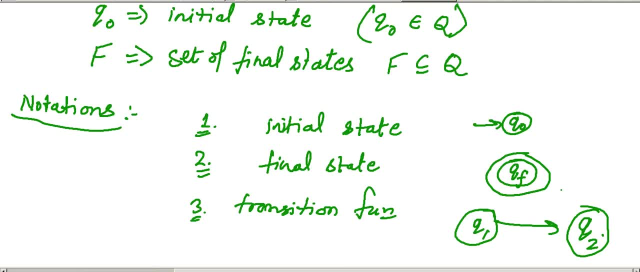 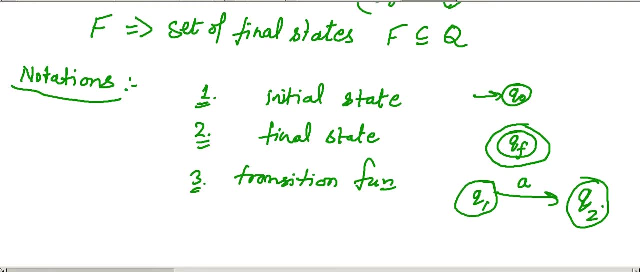 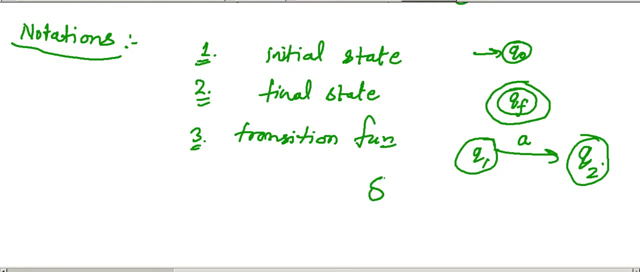 So this is the transition function, but it is expecting a reading, a symbol A from the input tape And then It's going to the Q2 state. So it can be represented as This: data Okay, And this Q1 state. 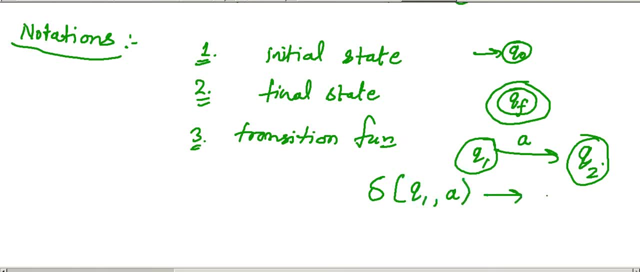 By reading a symbol, A, Going to this state with it: Q2.. So In the previous paper that was held in February, they have asked one question In which they have Asked you to draw a diagram using. They have given you a diagram and then asked you: 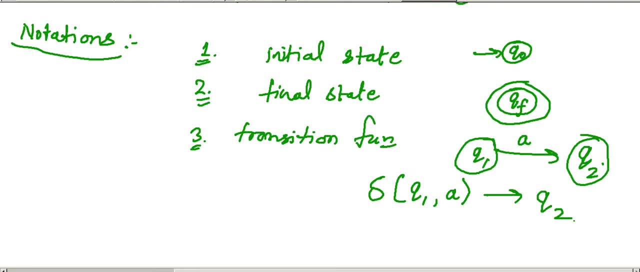 To, To summarize Those, Those, Those diagrams into a transition function. So Okay, So, these are the symbols and you must go about these symbols Before, Before Creating or designing a deterministic finite automaton. So Okay, So. 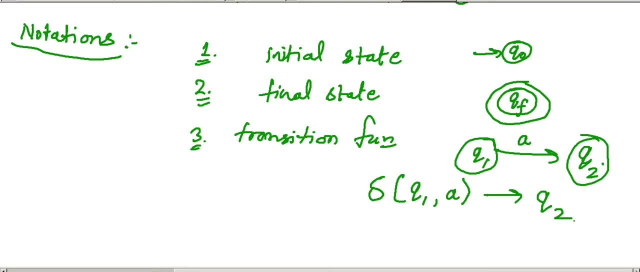 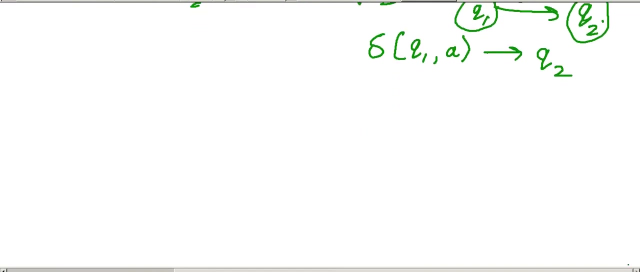 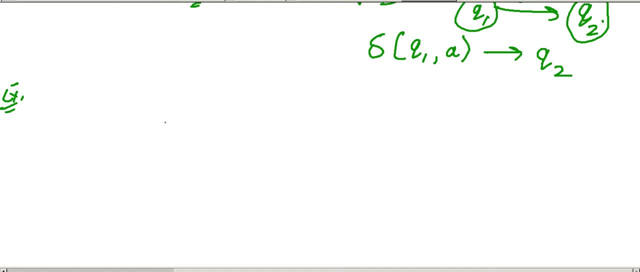 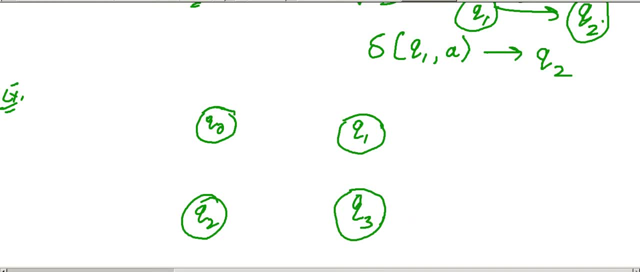 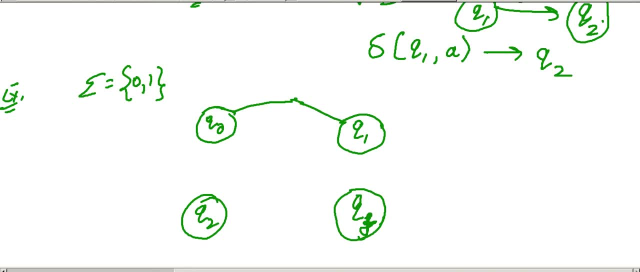 reading a symbol- Q0- and then going to the Q1, and Q1 is also reading 0. then going to Q0.. Q0 is your initial state and is represented by this symbol, and Q1 is reading 1 and Q is also reading 1.. 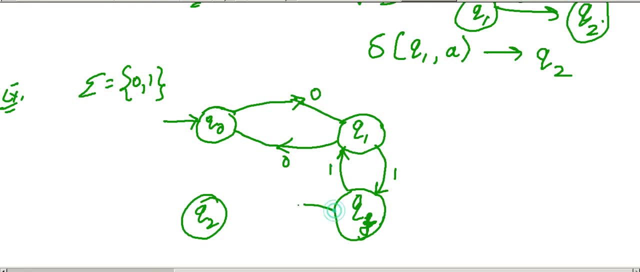 And these two are. so I will explain it right: This is 0, 0.. And again here we have: this is 1, 1.. So what does it mean? that they are asking you to create a transition function for that, and 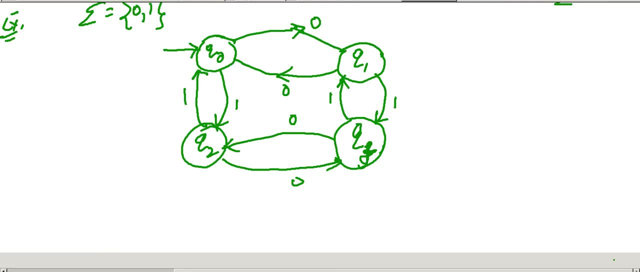 create a transition table actually. So how you can do that? So you have to draw it like that. So we have these symbols 0 and 1.. We have these states Q0,, Q1, Q2 and QF, And at Q0 we are reading 0 and reaching 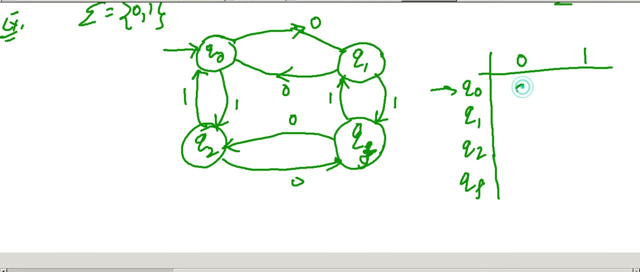 to Q1.. Okay, sorry, Reaching to Q1, and when we are reading 1, it is going to Q2,. right, It is going to Q2, so we will write Q2.. Now, from Q1, we have two transitions. If we are reading 1, then it is going to QF, So by reading, 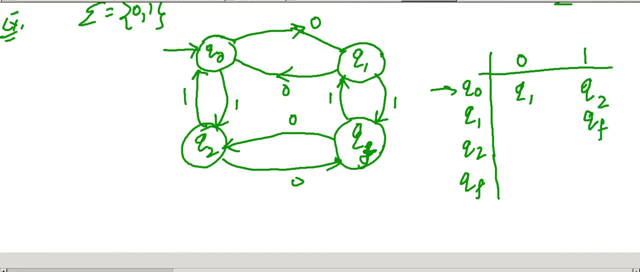 1, it is going to QF, And by reading 0, it is going to Q0. And at Q2, at this state, if we are reading 0, then we are going to QF, Right. And if we are reading 1, then we are going to Q0, right. And at QF, we are reading 1, then we are going to Q1. And if, at this state, we are reading 0, then it is going towards Q2, okay. 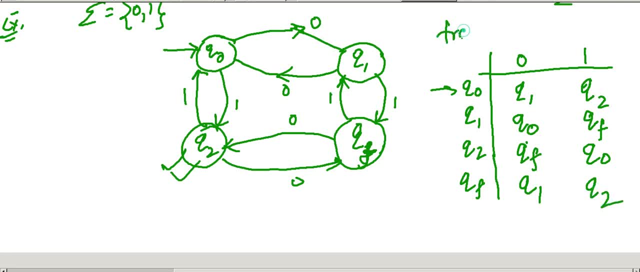 So this is your transition functions- right, Because it shows that how these transitions are happening. okay, And in exams they ask you to. they have given either this graph- okay, This graph is nothing but a deterministic, finite automata And they will ask you to draw a table of transition functions or, if they